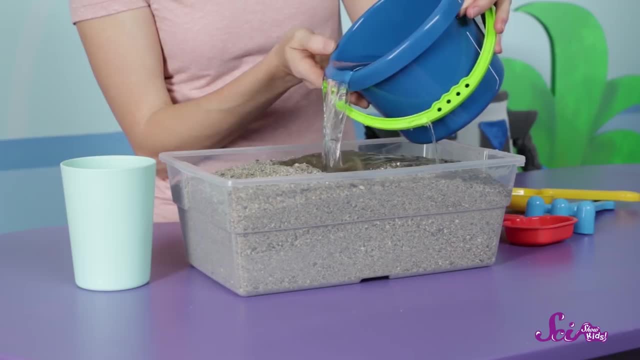 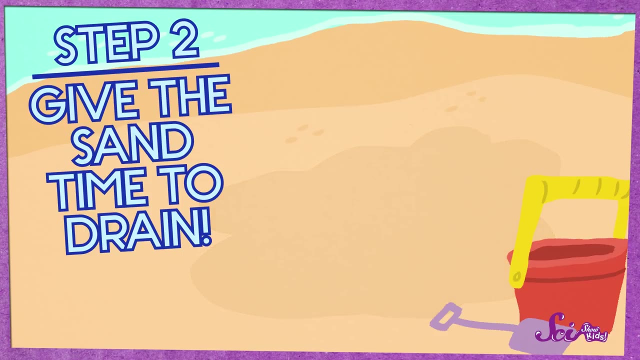 fall apart. So make sure you mix plenty of water in with the sand that you're going to use to build your sandcastle. Step 2. Give your sand a way and some time to drain. Draining the sand means making sure there's not too much water in it. 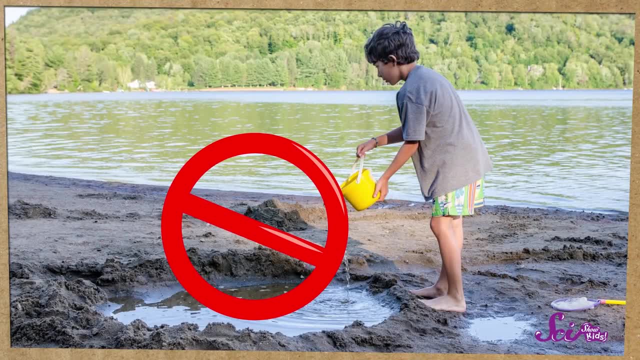 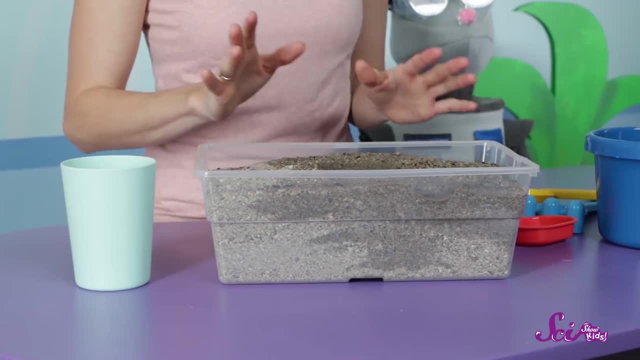 If it starts to look more like soup, that means there's too much water for those little bridges to form And the grains of sand won't fall apart. So you should let the extra water drain from the sand before you start your castle. That might mean using a tool with holes in it so the extra water can get out. 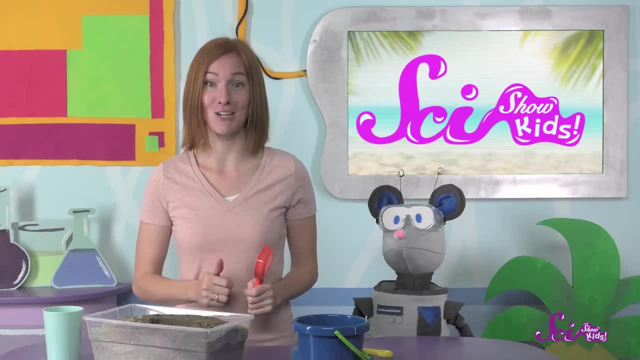 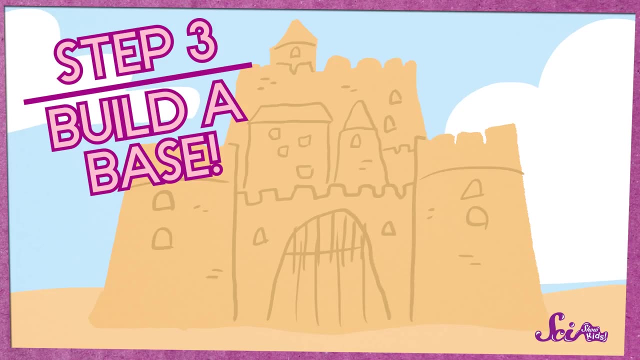 Or you might just want to let your sand sit for a few minutes before you get started. Once the extra water is drained out of the sand, you're ready to move on to Step 3.. Make the castle's base. Every sturdy building, whether it's a skyscraper or a sandcastle, needs a sturdy base or bottom. If the bottom isn't strong enough to hold it up, then you need a sturdy base. If the bottom isn't strong enough to hold it up, then you need a sturdy base. If the bottom isn't strong enough to hold it up, then you need a sturdy base. 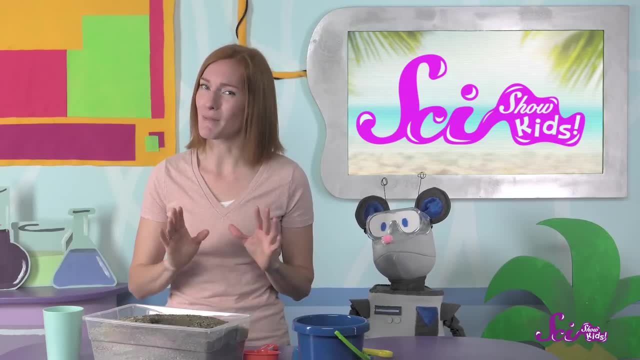 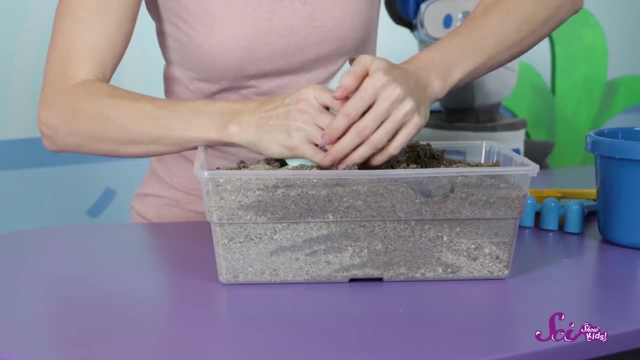 If the top isn't strong enough to hold it up, then you need a sturdy base. A good sandcastle base is made out of tightly packed sand, so if you're using a bucket or a cup, make sure you press on the sand to pack it in tightly. 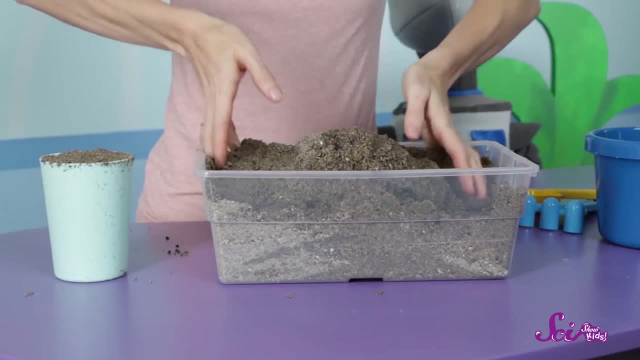 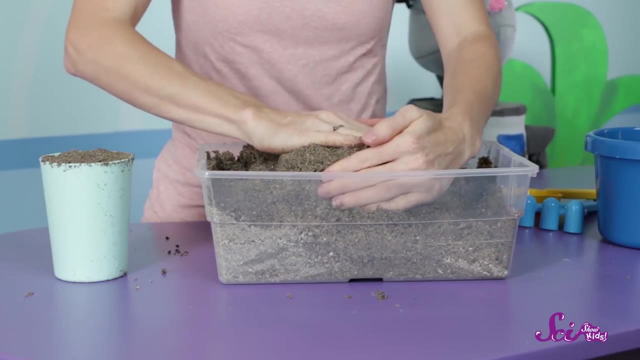 And if you don't have a bucket or a cup, no problem. Just make a pile of sand and press on it as hard as you can. Then add more sand on top and press again. Do this over and over again until you have a nice big pile of sand. that's tightly. 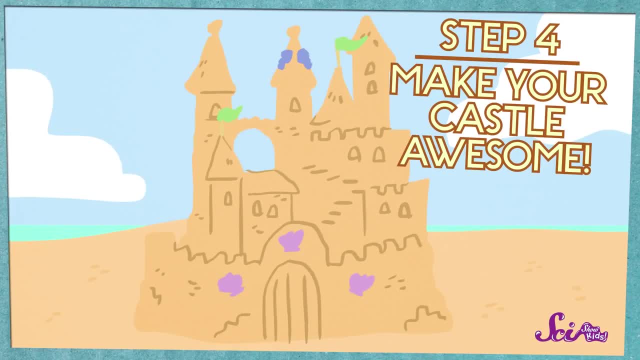 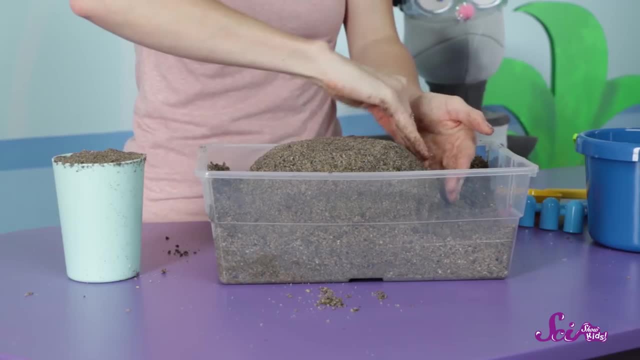 packed. Step 4. Use your imagination to make your castle awesome. Step 5. sturdy base. you're ready to shape your castle. You can use your hands and fingers to shape the walls. Then you're ready to add towers, seashells or anything you can imagine. 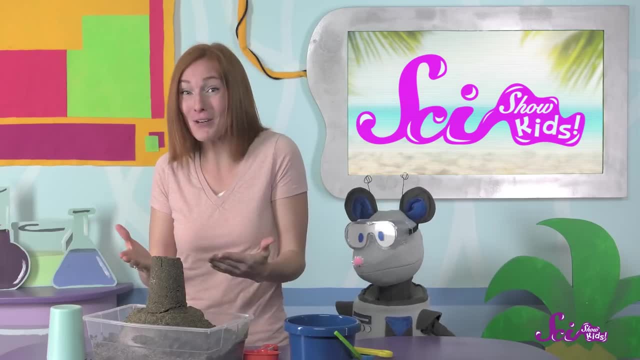 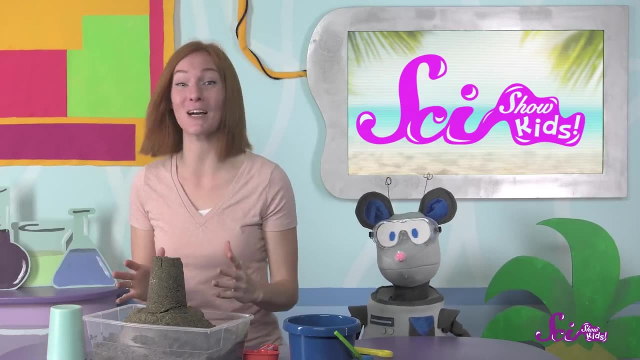 Just make sure not to add too much sand on top of your base or your castle might crumble. And no matter what kind of castle you build, don't forget to have fun while you're doing it. I'm excited to keep working on my castle and make it even more awesome. 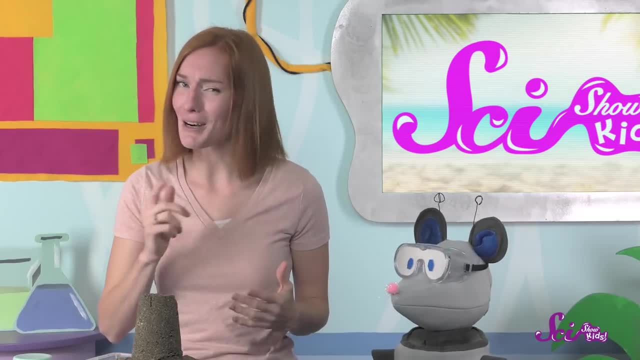 If you build a sandcastle of your own, we'd love to see it. Grab a grown-up and send us an email to kids at scishowcom. In the meantime, don't forget to hit the subscribe button and we'll see you next. time here at the Fort.